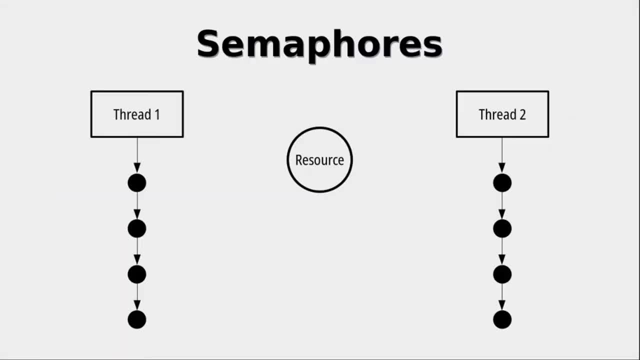 In this video, we will take a look at semaphores. Now, in the last video, we have seen multi-threading and concurrency, and we have seen what can happen if multiple threads have a shared resource that has no synchronization behind it. Now we solve this problem by using mVars and using channels. 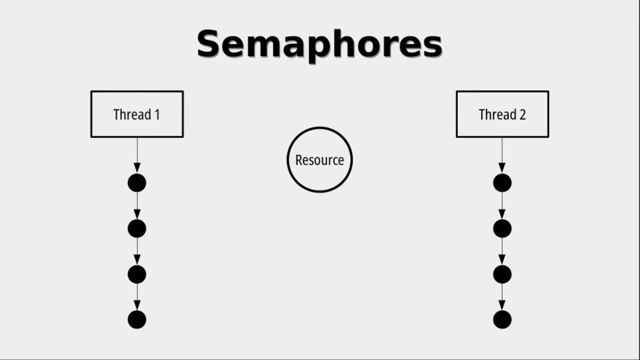 but now we want to do that with semaphores. Okay, so we have the following setup where we have two threads and one shared resource. In this case, every thread has its own control flow and we have a scheduling so that first thread one goes first, then thread two, then thread one and 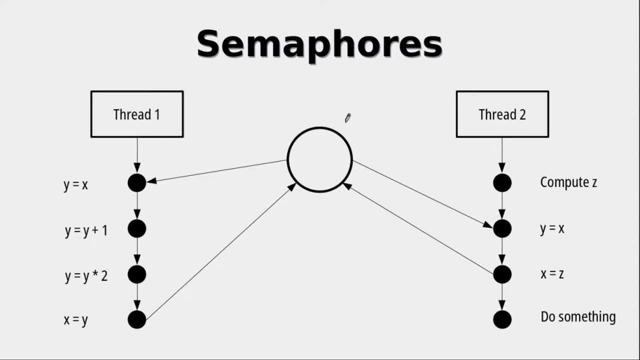 then thread two. That's the scheduling that we will use for now and the shared resource. we will now call x. Okay, so let's assume that it has some initial value, let's say four, and what we're going to do is transfer it to the resource. Now we're going to call other blue threads. 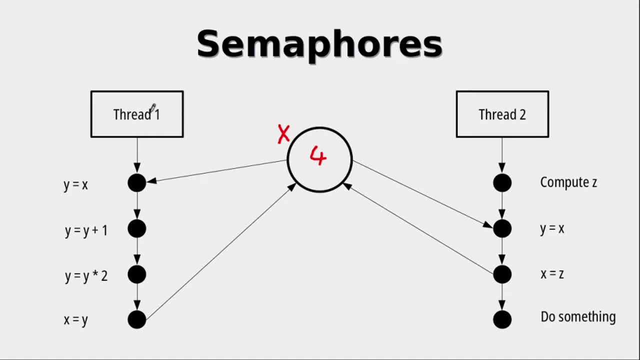 okay, and we're going to Shakespeare the new string and take this one. so in this case we have, we're going to take every shared resource and the shared resource and then take this one in here. Let's simulate this, Okay. so threat one goes first and saves X as a local variable. Y. 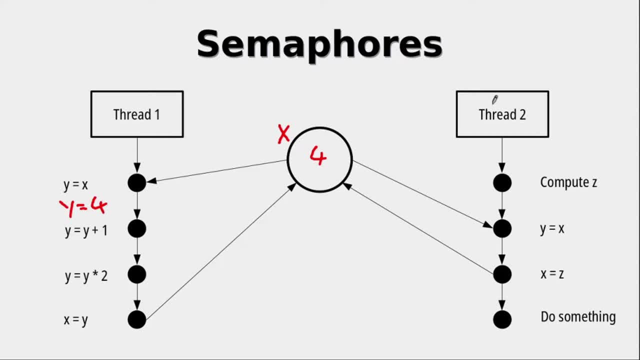 so Y is four. Threat two does some computation and computes a Z. Now, this Z, let's just set it to one, okay. so Y does some other calculations and calculates that Y is five. Now threat two tries to get hold of the shared resource, which it can, of course, and saves. 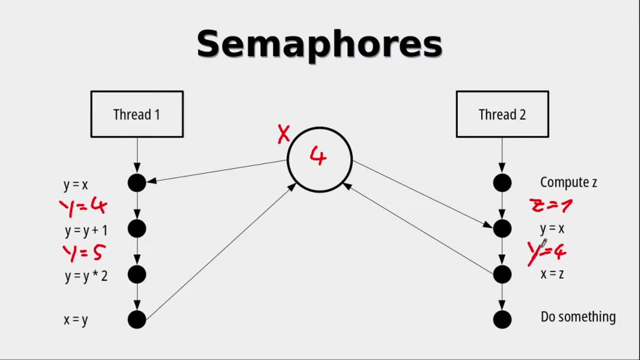 Saves the shared resource as some local variable Y. Of course, those two Y's are not the same. This is the local Y for threat one. This is the local Y for threat two. Okay, so now threat two has a go and does some more calculation. Now, what threat two tries to do is the: 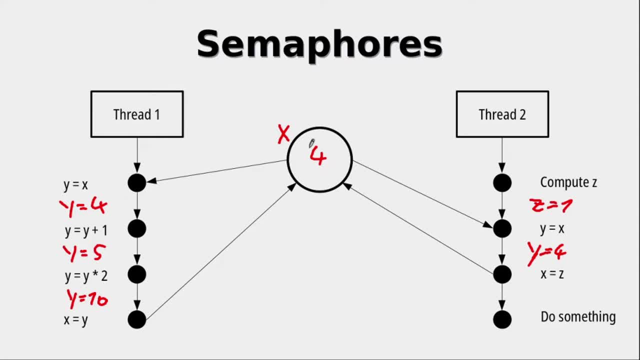 Threat two does some more calculations and computes a Z that it had before. it will now store into X. So now, of course, nothing changes when it comes to the values, but this four is now a one. Okay, and now threat one Does the same thing actually, and it tries to store. 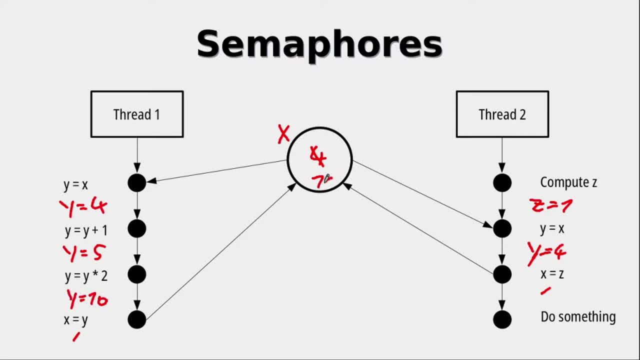 That the value of Y into X, So now it is actually 10. and now threat two does something. but the problem, of course, is that Threat two thinks it successfully stored whatever the value it tried to store. So it tried to store the value one it tried to. 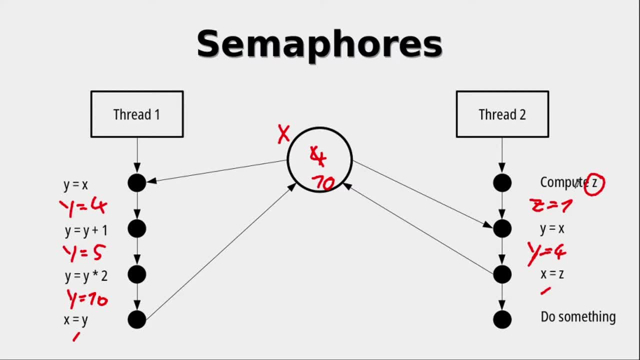 Store the computed Z. but that is not the case, since we had a race condition here where threat one over well did some overwriting and basically deleted the result of threat two. This is, of course, the the well the, the trivial example of a race condition. This is a huge problem for any concurrent program and we want to 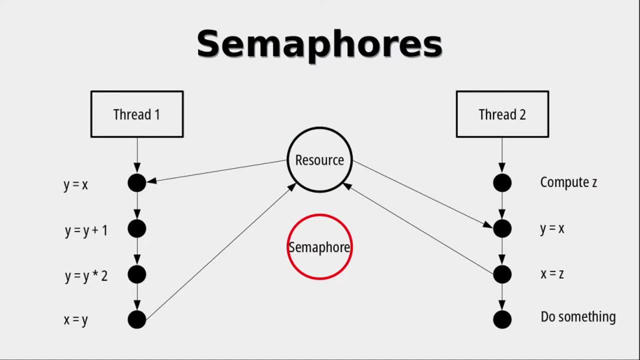 Well, we want to synchronize this by using a semaphore. now, What is the semaphore? that really depends on the system and the language you're looking at. in Haskell, Again, our shared resource is called X and our semaphore here. That is just some counter that. 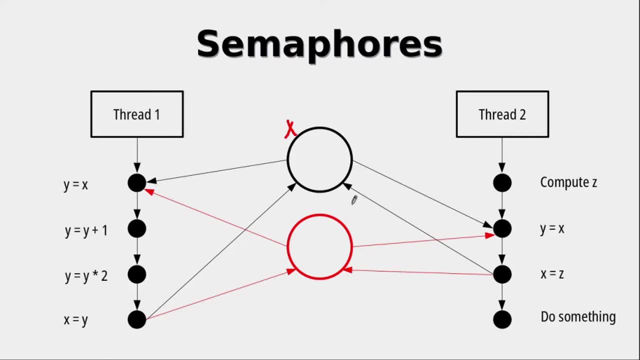 Has values from zero to infinity, basically. So in our example, we want to set the initial value of the semaphore to one, because how this will work Well is basically the following: when a threat wants to work with the resource, It has to acquire the semaphore. this means that it basically: 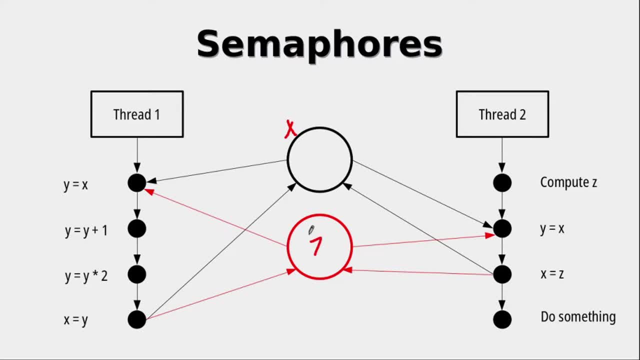 Subtracts one from the value of the semaphore and then does whatever it wants to do. if the value is already zero, Then there is nothing to subtract, Since the semaphore cannot be negative. So then we are waiting. Let's look at this in action. We will set X to. 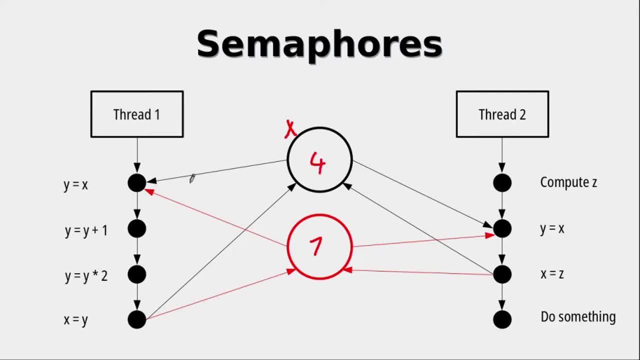 Four again. okay. So threat one goes first and it acquires the lock of the semaphore. It's very important that this has to be done before We are working with the resource. So now, this is not one, This is zero. Okay, so now we set one. 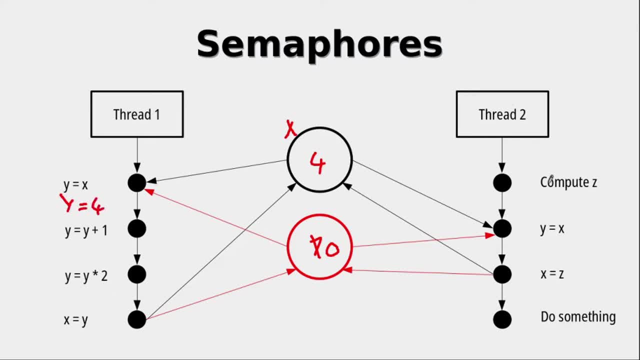 To X. So Y is for threat to compute set. Let's again Say that set is one. Now we do some calculation in thread one again. and now threat to tries to acquire the semaphore in order to well have some control flow here. but it can't, because the semaphore 0, so now threat 2 is actually. 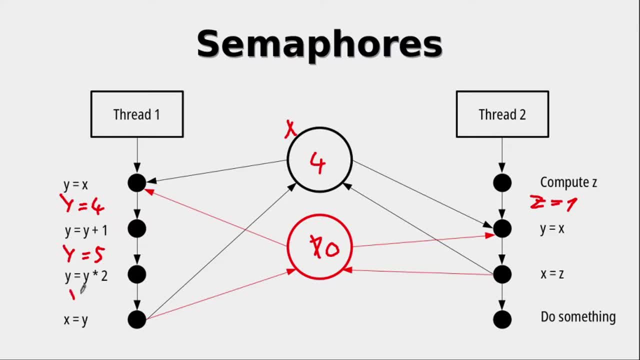 waiting. So now threat 1, Thread 1, is going again. thread 2 has to wait here, and now thread 1 can actually store its value 10 into our shared resource here. Now the important thing is that it has to release the semaphore again. 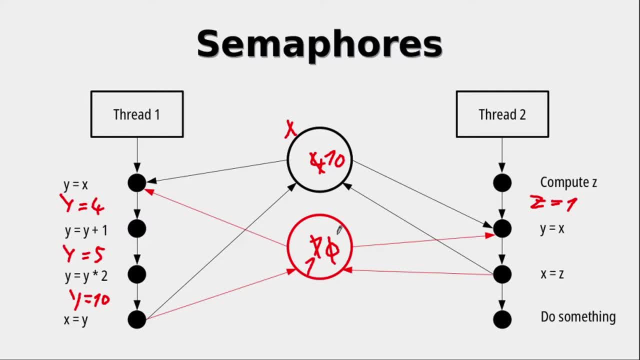 So now it releases it and stores a 1 into the semaphore. Now thread 2 can go. So in this case, y is now 10 and the semaphore is 0 again, and I'm running out of space to draw here. So now of course, thread 1 is finished in our case. so thread 2 still has to do some stuff. 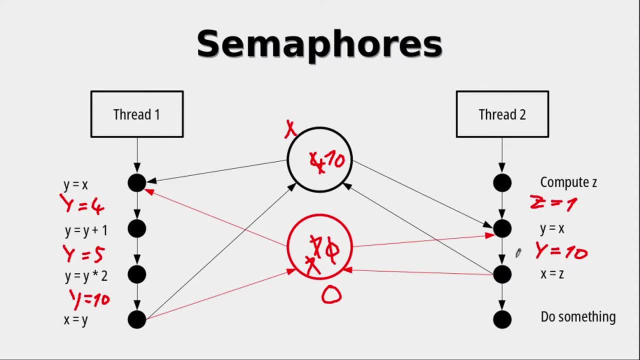 In this case it does the swapping of y and z. So now it stores 1 into the shared resource and that's about it. It releases the lock again, so it releases the semaphore again. so now the semaphore is again 1 and we're finished. 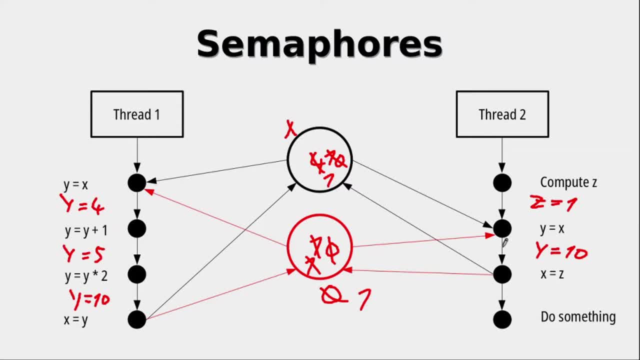 Now, of course, we did some synchronization. When a thread wanted to work with the shared variable or the shared resource, it had to acquire a lock via a semaphore, and this is hugely important for multithreading. So let's look at how semaphores are implemented in Haskell. 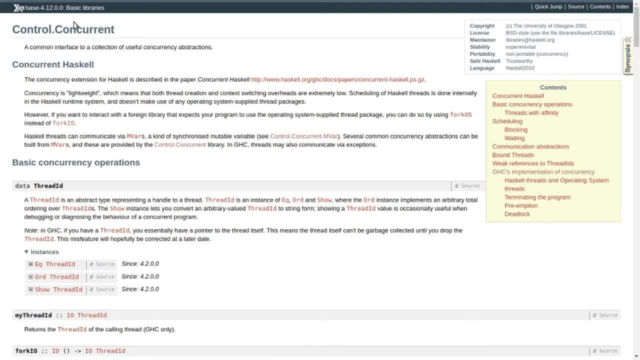 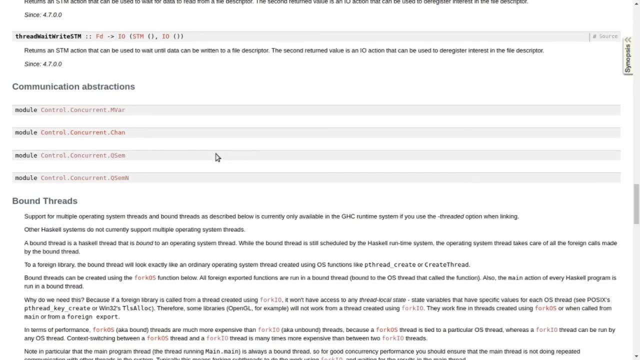 Okay, so we are in the documentation of controlconcurrent. Let's look at the data types that we might use in order to have semaphores. Well, in the last video, we actually used channels and mmars in this sense that we want to use. 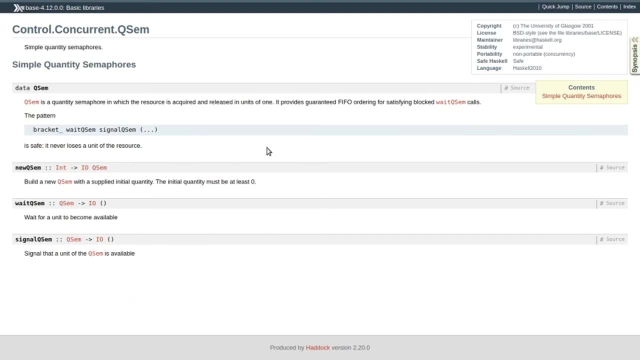 a semaphore, but now we actually use the correct data type. So the correct data type is QSem and QSemN. QSem is a quantifier. This means that it behaves just like the example that I showed, where you have some semaphore. that is basically a counter. that cannot go negative. 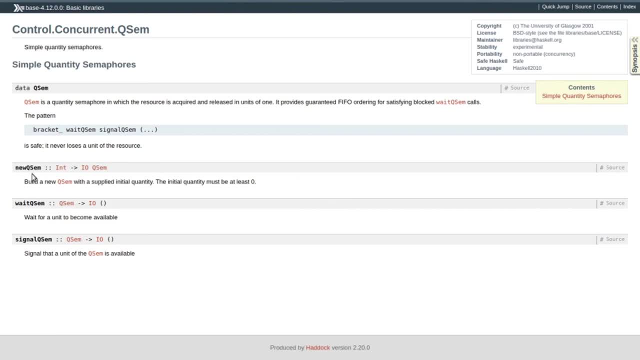 Now you make a new semaphore with new QSem and you supply it an int. This means that you have to have some initial quantity. It must be at least 0, and then we have waitQSem and signalQSem. WaitQSem, of course, decrements the semaphore by one, and signalQSem signals to the semaphore. 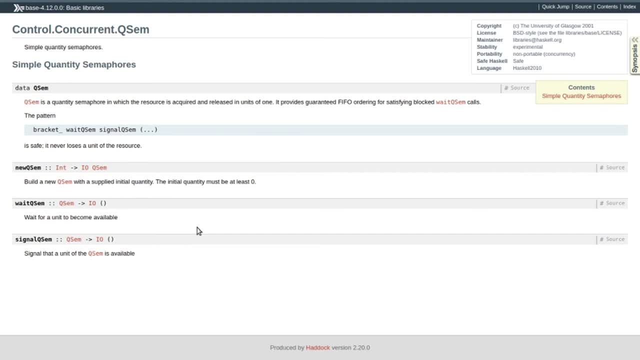 to increase the value by one, to increment it. Of course waitQSem is blocking, and this is very important. Now, another important thing is that there is no upper bound to the quantity of the semaphore, So it can go to well whatever high number you can think of. 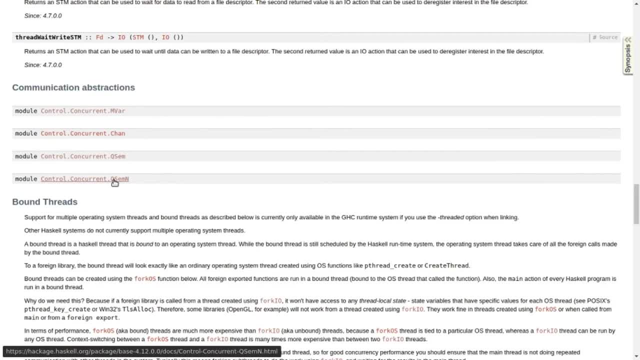 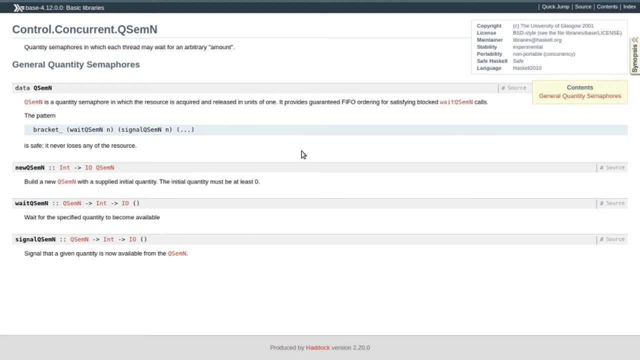 So it can go to well, whatever high number you can think of. So it can go to well, whatever high number you can think of. Then there is basically a sibling to this data type called QSemN. It works just like it worked before, but now waitQSem and signalQSem actually can increment. 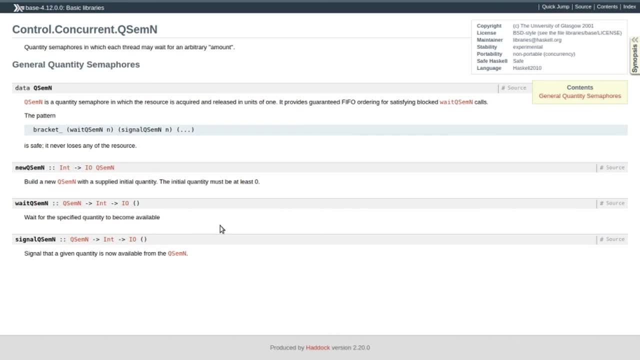 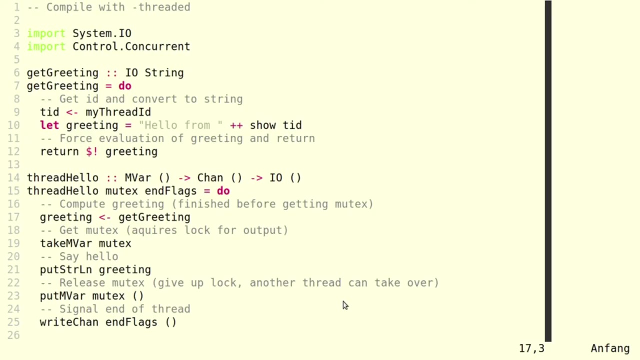 or decrement by more than one. This is very helpful if you have to. well, we will see this in a second. if you have to wait for multiple things happening, Okay, so let's look at an example. Okay, so here we are, back in the code of the last episode. 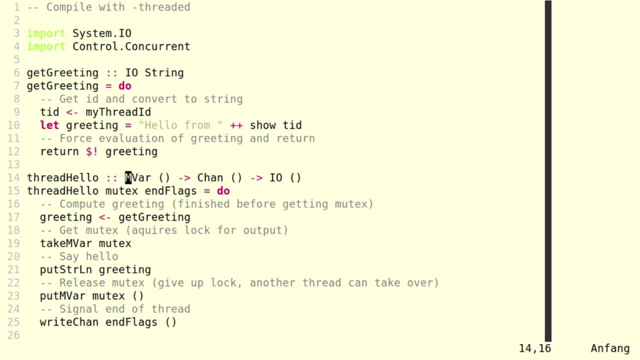 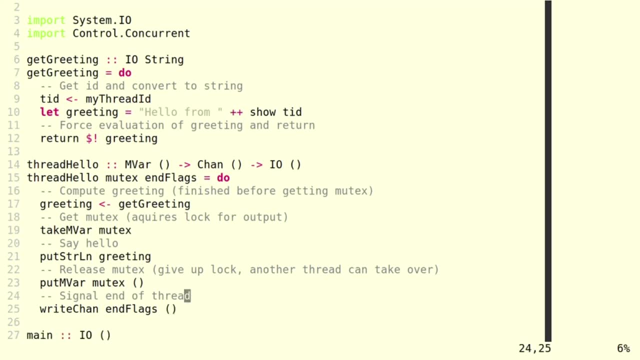 We want to rewrite this: instead of mMars and chans, we want to use QSems now. Okay, so let's think about this: We had one mutex that was giving exclusivity, mutual exclusivity, to the standard output. So how would you implement that? 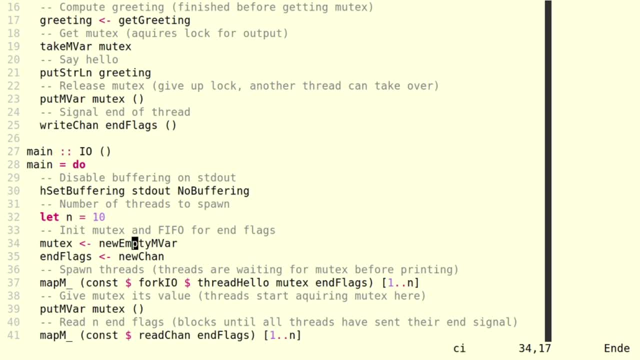 Well, of course We can do it with a single QSem. So now we create a new QSem with initial quantity zero. This is very important. of course, There shouldn't be anything in the mutex, since after the creation of the threads we want. 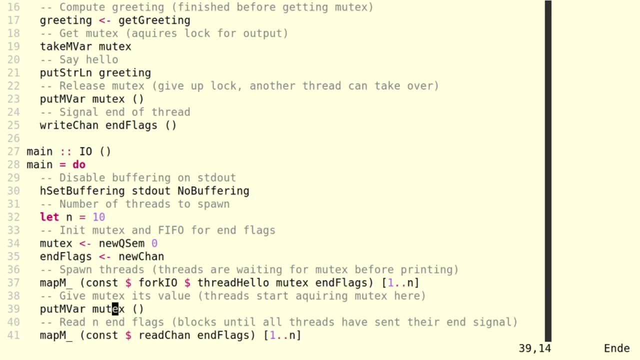 to signal that they now can start well printing something to the screen, And that's also what we want to do. What we want to do in the main is we want to signal the QSem Okay, Or we want to signal to the mutex that it now has the quantity one. 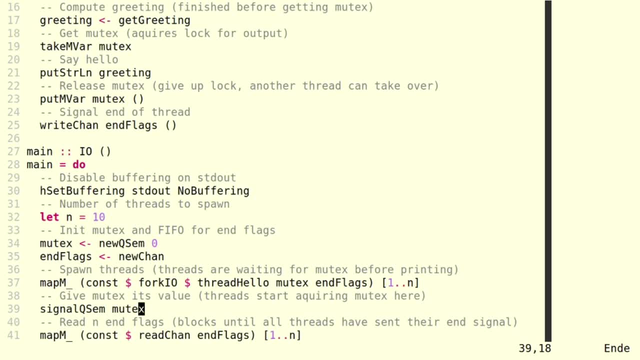 Now it's very important, of course, that if we have a mutex, the quantity can never go over one. It should never be two or three, since then multiple threads can acquire it. So that is something that we have to make sure. There is no well automatic way of doing that. 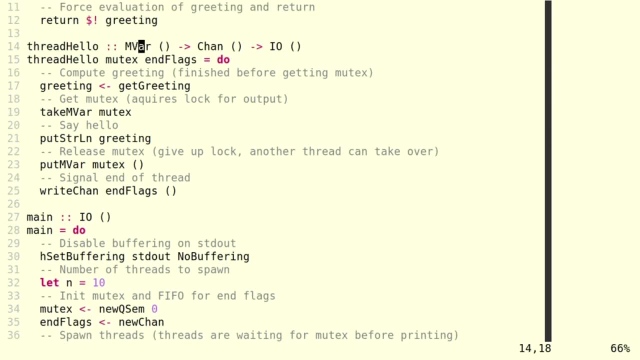 Okay. So now of course, we have to change our thread. hello The mVars. Okay, The mVar is now a single QSem and we have to change the functions that we used. So instead of taking something from an mVar, we now wait for the QSem. 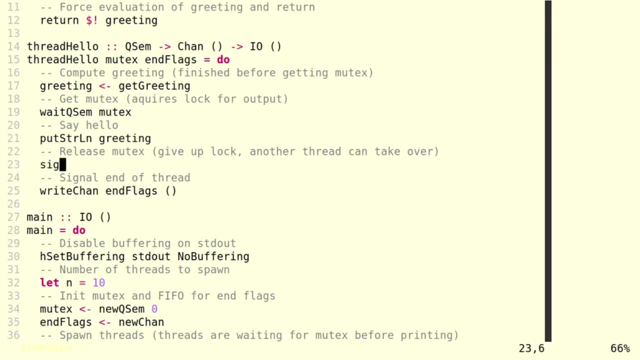 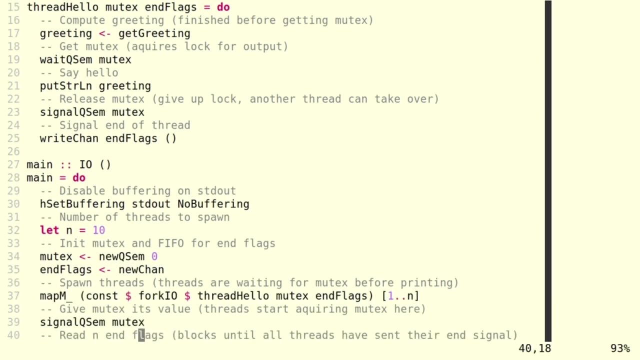 And instead of putting something back into it, what we do is we signal the QSem And that's about it. But now the question is: how do we handle the end flags? Now, of course, our main function in the end flags is the QSem. 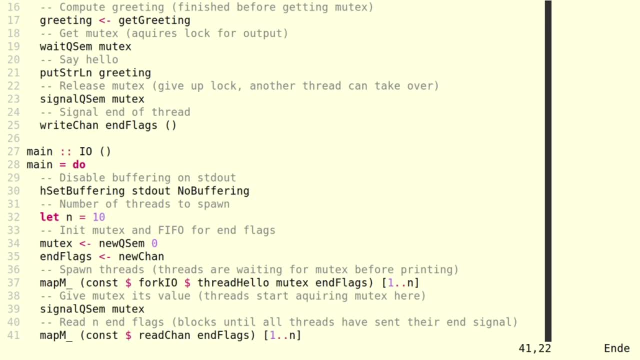 And that's about it. But now the question is: how do we handle the end flags? And that's about it, And that's about it. So now the question in the end wants to read: n well, units of data from this channel in order to understand that every threat has finished. 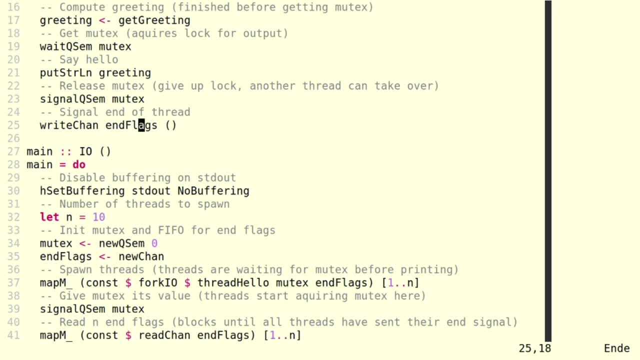 Since every threat signals its end with one unit of data in this channel. Now we can implement that with this QSemn. Because waiting for the end flag? So let's just, let's just use a QSemn Again, with initial quantity zero. 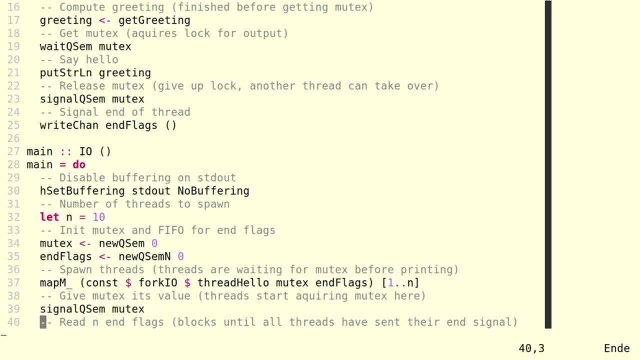 because this whole call can actually be done by waiting for the qsemn, which are our n-flags, and with the quantity n. so this means that we wait until the n-flags, until the, the semaphore n-flags has the quantity n if we start with 0 and every thread just supplies it the quantity. 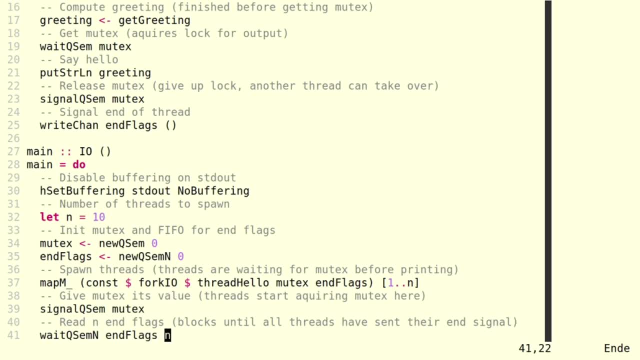 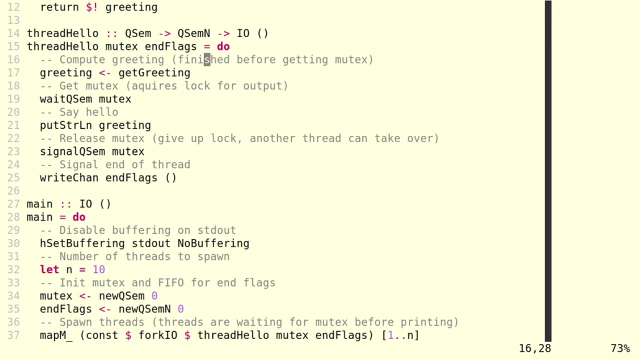 1. then of course, we know when every thread has finished once. this is n okay. so now we have to do some little changes to our thread function. so let's do that, and the only change we have to do here is the right chan now, of course, is a signal qsemn to the n-flags with the value 1. 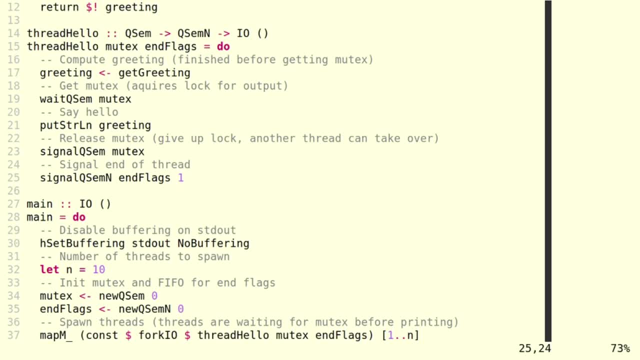 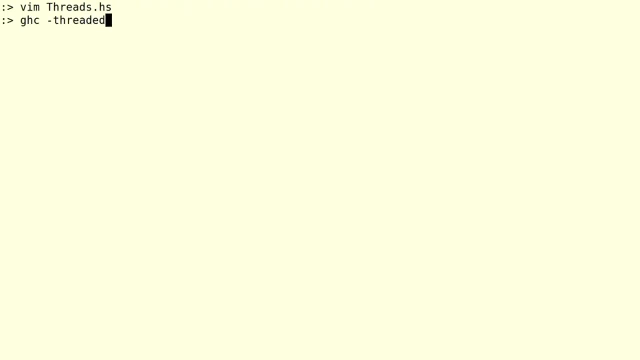 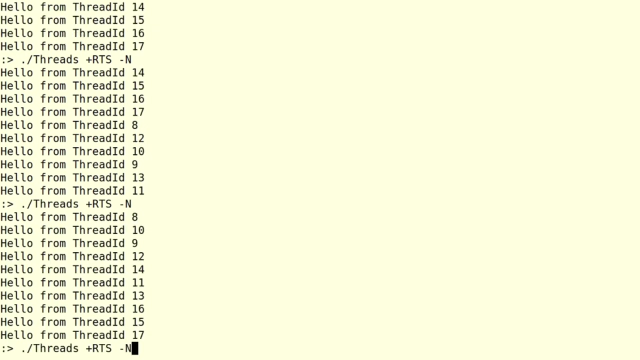 test this, shall we? of course, we have to compile it with the threaded flag and, yes, we're compiling it, we're linking it. now we can call the program. of course we want to do it in a multi-thread way and, as we can see, it is the same result that we had in the last episode. it works perfectly. 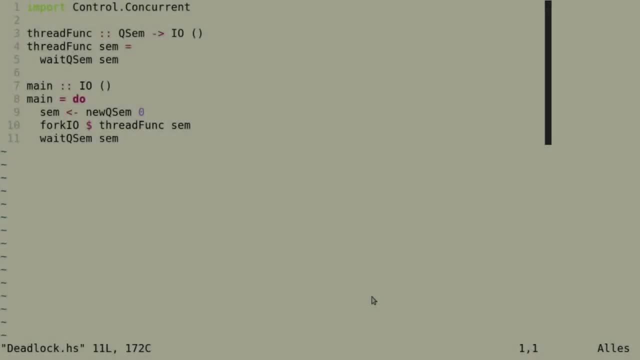 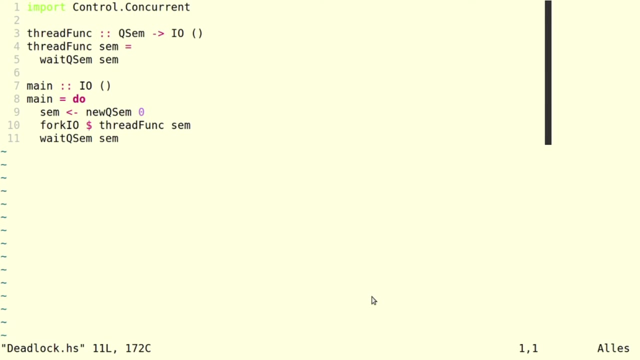 like a charm, But it isn't all that nice. Semaphores have a huge problem Now. semaphores are so-called locking, synchronization mechanisms: Locking because we acquire a lock for a certain resource. Sometimes this resource is the semaphore itself. This is a huge problem, since you cannot 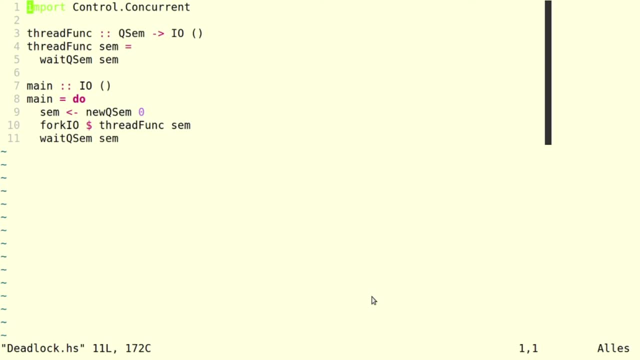 really make sure automatically that you will always give some quantity to the semaphore. What if a thread is waiting on a semaphore and another thread that needs to signal to the semaphore is crashing? In this case the semaphore will never be signaled again and every thread is blocking. So this is a very trivial example where our thread function only waits for a 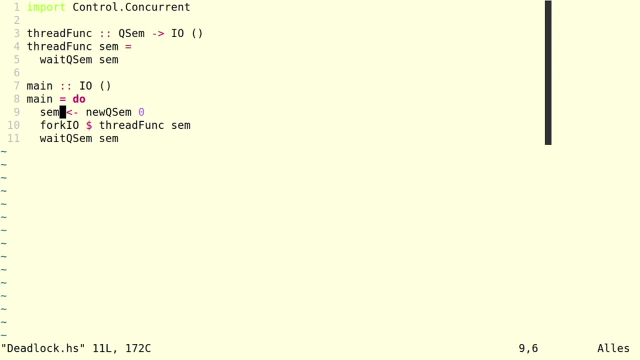 semaphore, And what the main IO action does is: it will create an empty semaphore, then forks the thread and then waits itself. So now both threads are simply waiting forever. Let's look at that in action. So we're compiling it and now we can run it And, as you can see, we get an error. 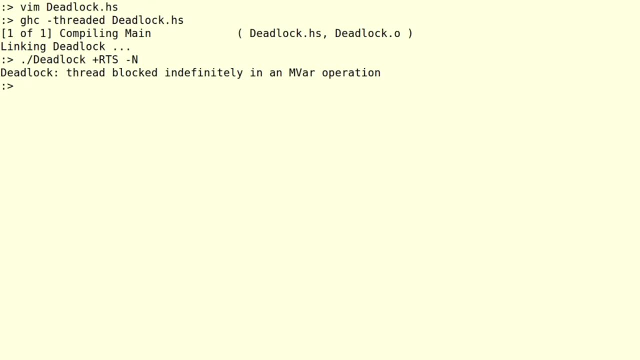 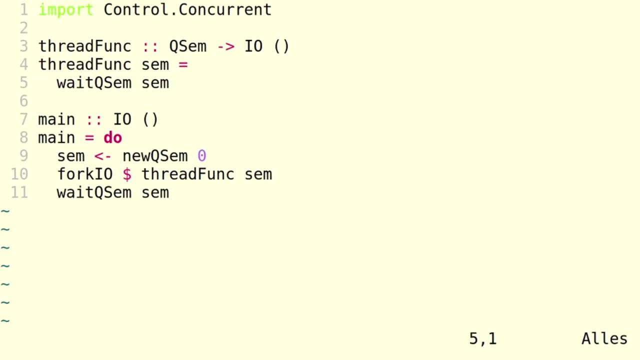 This is a deadlock error. Now, you're code should never produce this error. But now the question, of course, is: how do you make sure whoops, how do you make sure that this can never happen? And this is a very important question and also a highly debated research topic: how we can find out whether programs do not have